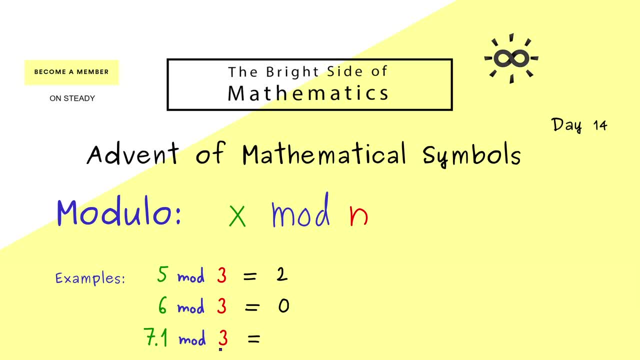 Also, here we find that the 3 fits 2 times into the number on the left hand side. Hence the remainder term is exactly 1.1.. So I hope you now know how this works. I like thinking of subtracting 3 so many times until something less than 3 remains. 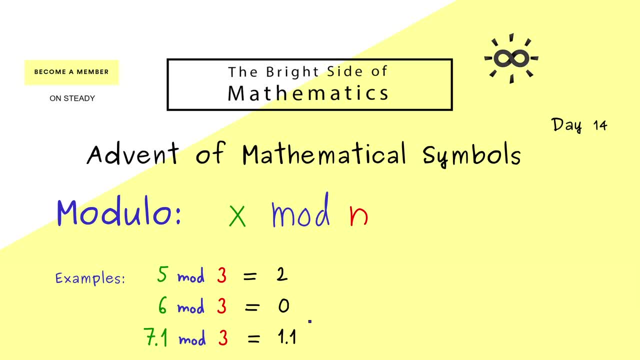 And the thing that remains Is exactly our result. So maybe I should also explain this with an example. So let's consider 9.7 mod 2.1.. So first let's subtract 2.1 here, So we get 7.6.. 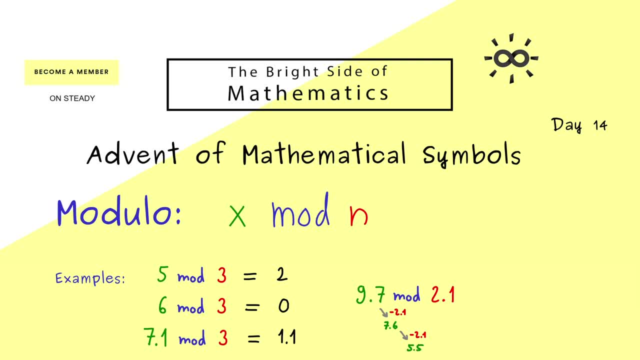 So let's do it again, And then we get 5.5.. Of course we do it again, And then we get 3.4. And then, in the last step, We finally get 1.3. Which is, of course less than 2.1.. 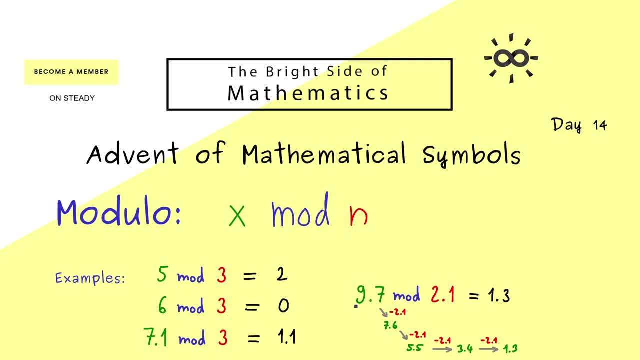 Hence. this is our result here, So this is how you can think of this, But the important thing is always remember It's the remainder term we want here: Hence. here for the definition, we could simply say: This is a number r And this number lies in the interval 0 to n. 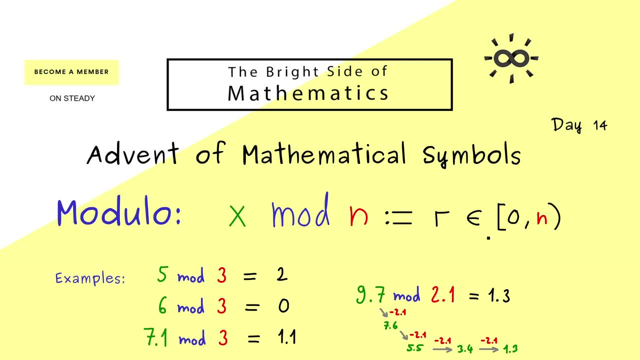 Where n is not included. However, of course, The remainder term could be 0.. Moreover, Now we also know how we get this number r, Because we can write x as a sum, Namely it's n times an integer. We can call q. 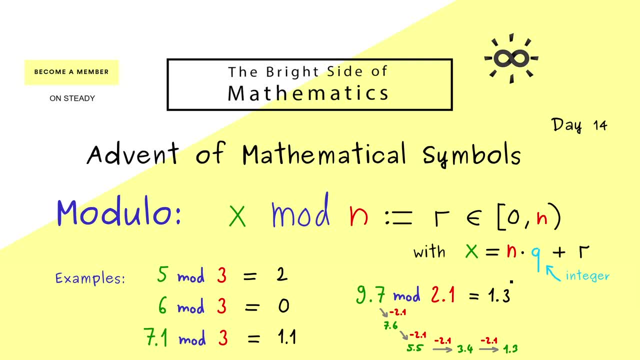 Plus the remainder term r. So you see, For our positive numbers x and n, This is exactly the procedure we explained before. Ok, Now for the end of the video. I want to show you how the modulo operator is included in python. 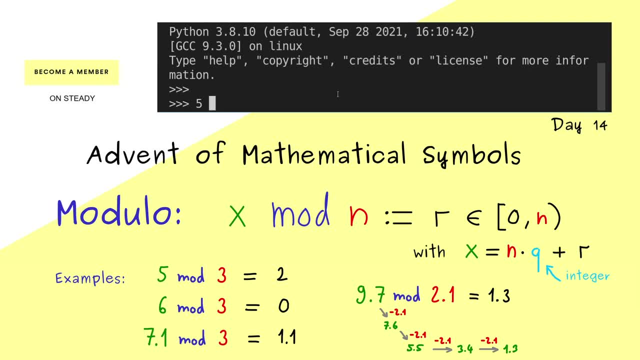 Indeed, This is simple. Instead of mod, We use the percentage sign. So you see, This is exactly what the modulo operator should do And, of course, It also works for our decimal numbers, As we had it before. However, As you can see, 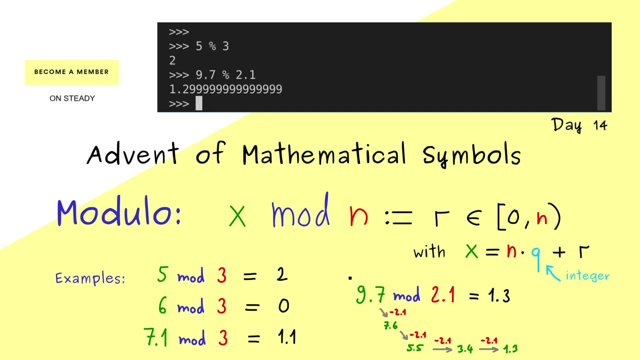 What can occur are some rounding errors. Ok, And with this, I hope I see you next time. Bye.